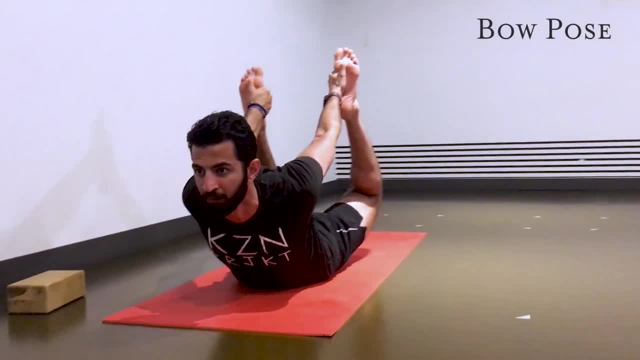 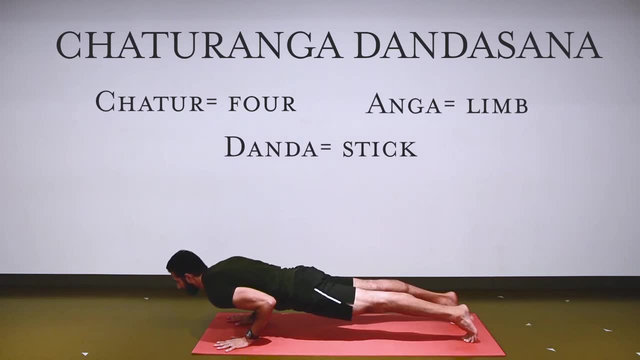 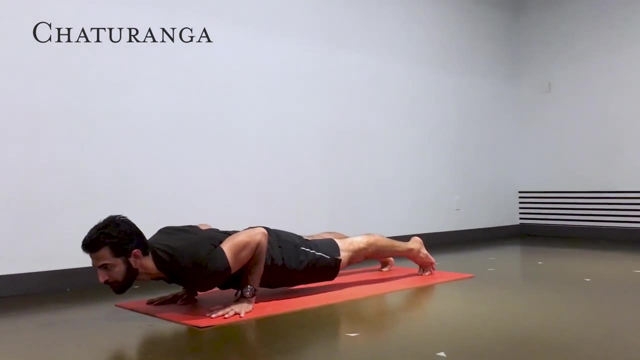 and building up tension just like a bow, And hence the pose is called that Chaturanga Dandasana Chatur for Angalim Dandasana. Chaturanga Dandasana, Also known as Yogi Bhujang Urdhva Mukha Svanasana. 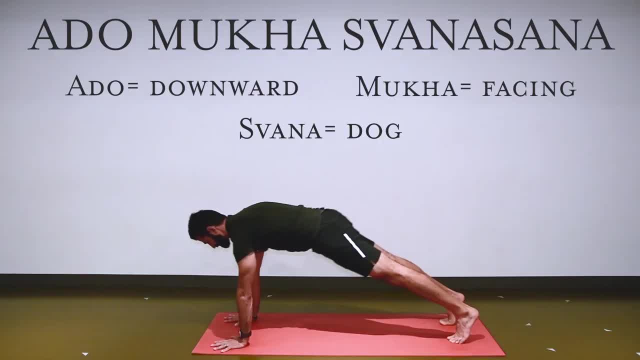 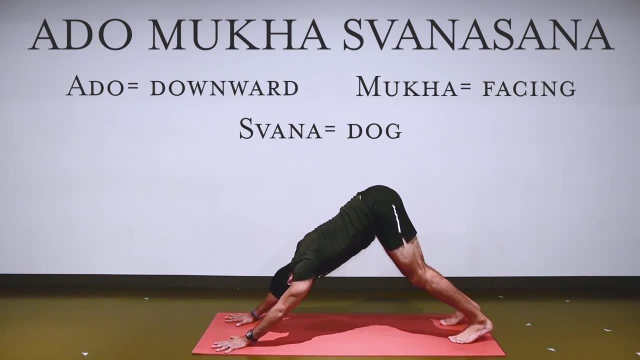 Urdhva. upward Mukha facing Svatna dog. Adho Mukha Svanasana Adho. downward Mukha facing Svanasana Dandasana dog A Thomuka Svanasana Tadasana. 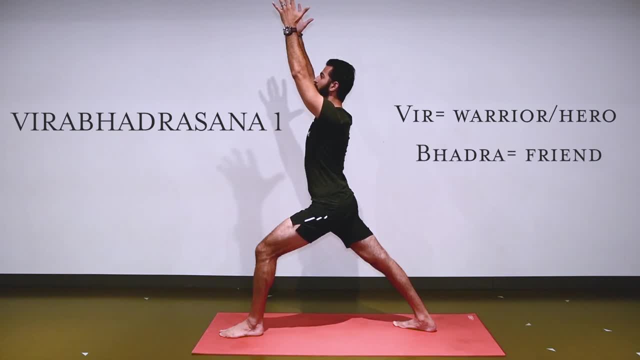 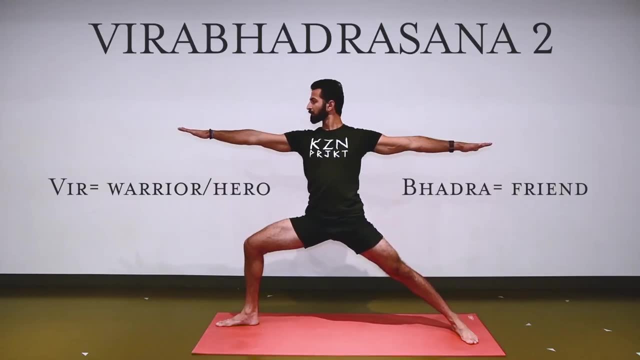 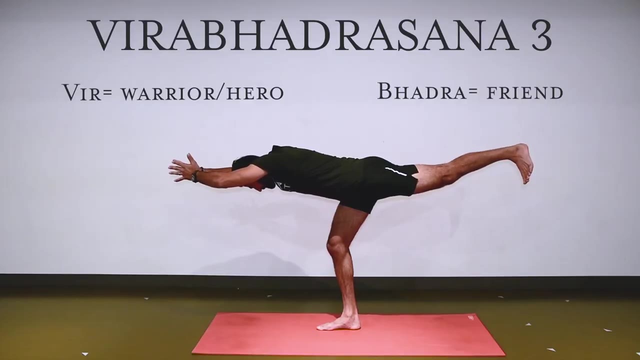 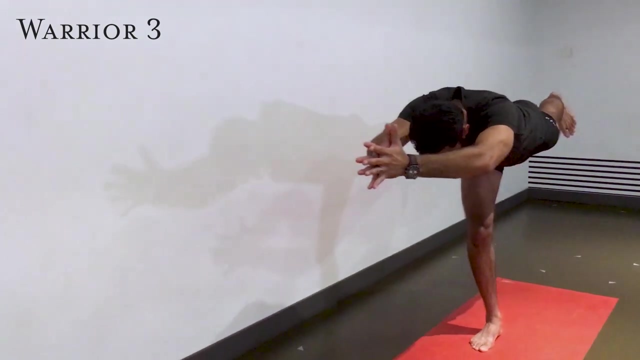 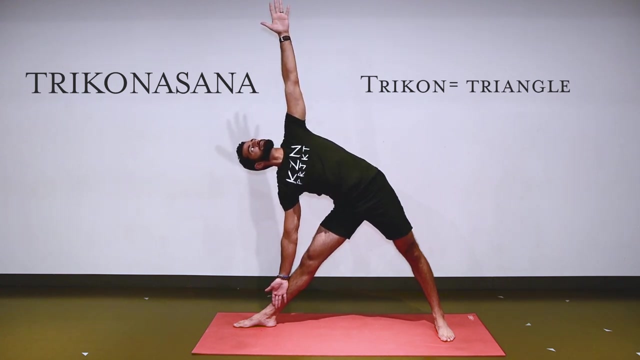 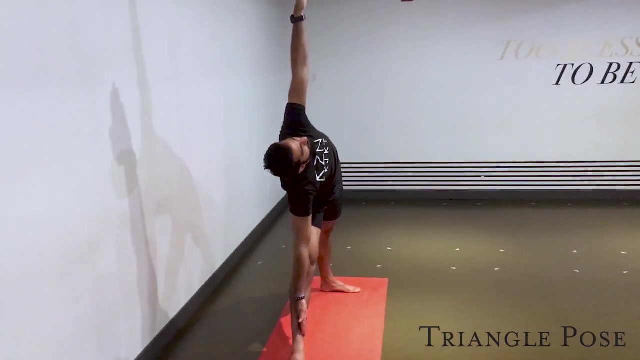 Veerbhadrasana, Part of the Warrior Family of Poses: Warrior 1, Veerbhadrasana 1 Or Veerbhadrasana 8. Veerbhadrasana 2. Virabhadrasana three. Trikonasana, Trikon, triangle Trikonasana. 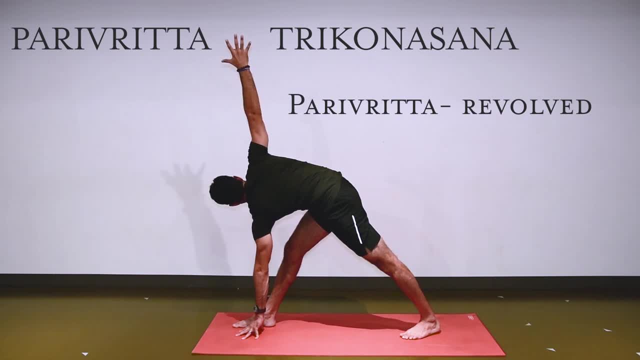 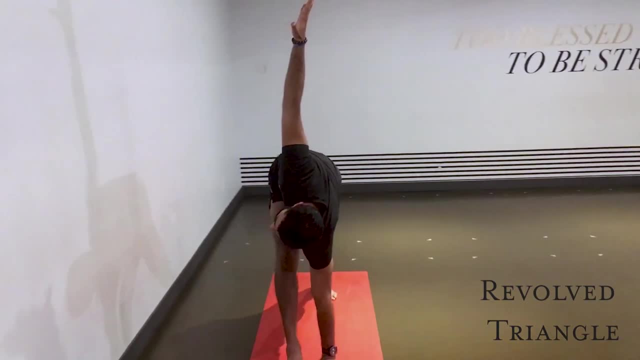 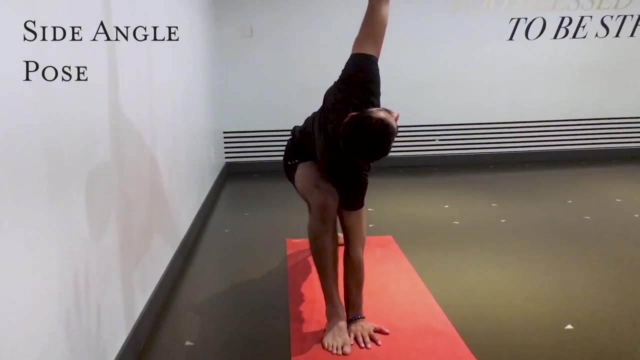 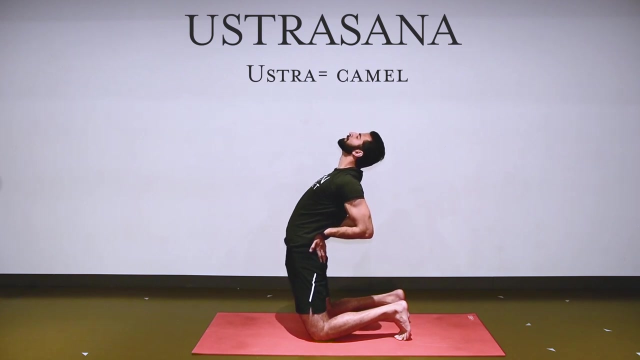 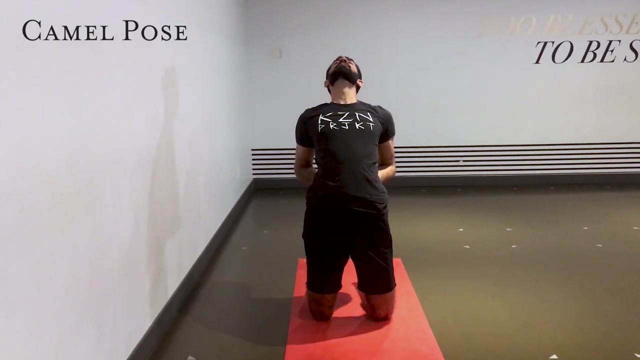 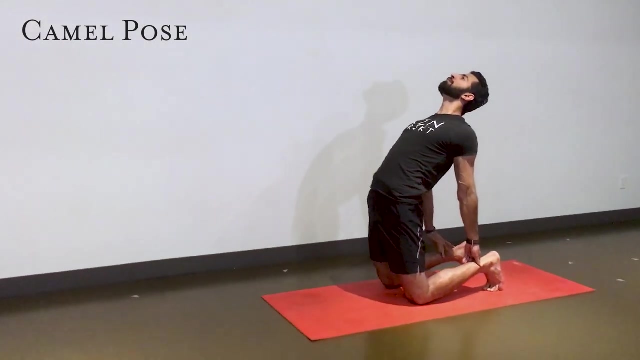 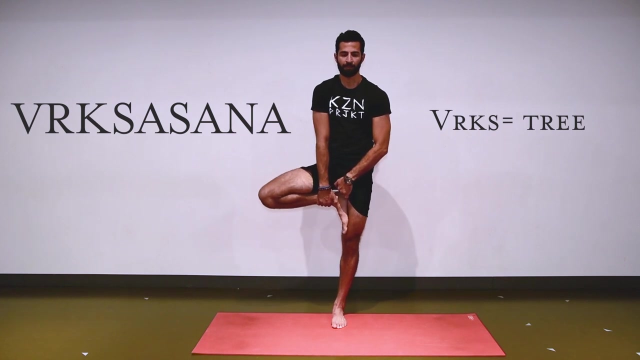 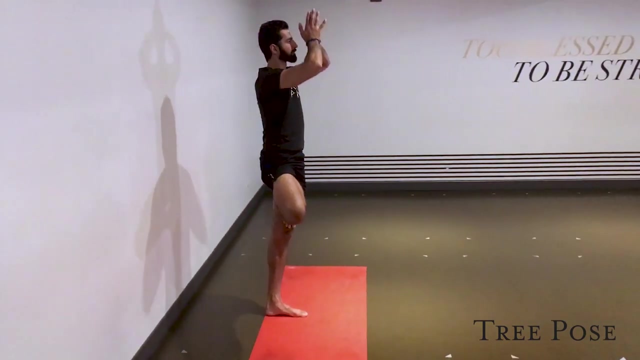 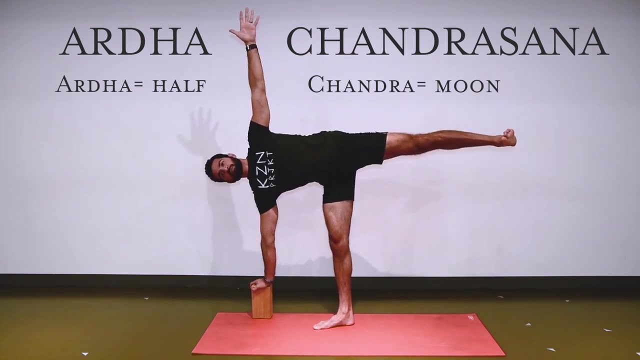 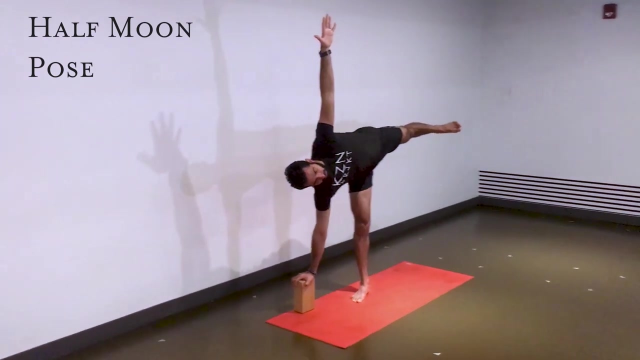 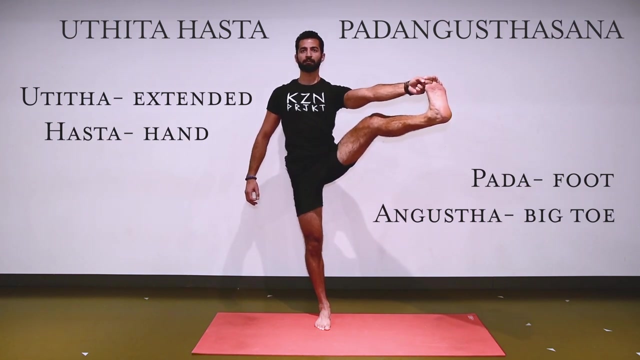 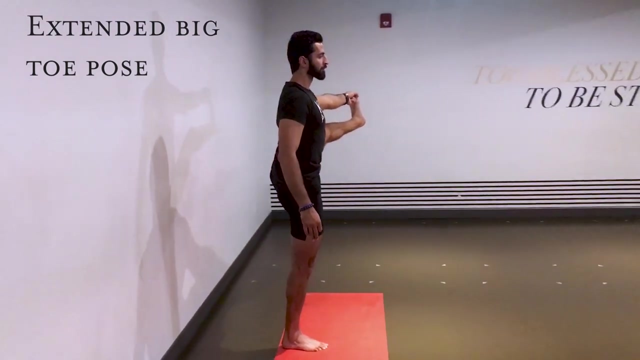 Parivritta Revolved Trikonasana. Parivritta Trikonasana. Parsvakonasana Ustrasana Vrikshasana, Vrikshasana Ardha Chandrasana, Ardha Chandrasana. Uthitha Hasta Padangusthasana, Uthitha Hasta Padangusthasana.